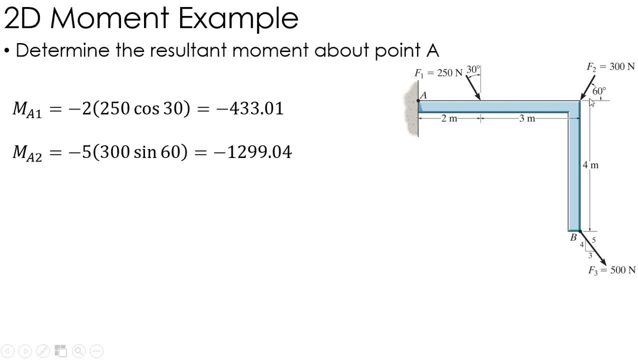 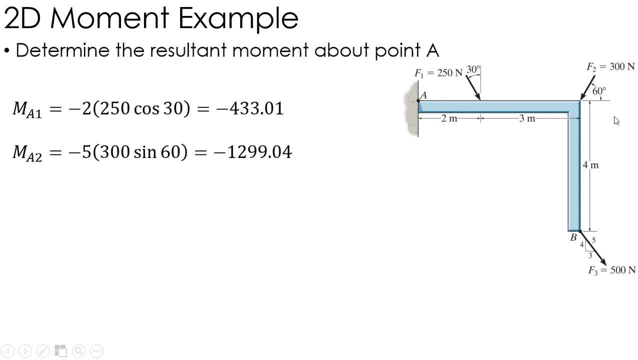 It has a distance, a moment arm of 5 meters. That vertical component acting down here creates a clockwise rotation as well. about point A. That's a negative moment about point A. Five feet away, Three hundred sine 60 is the perpendicular component. 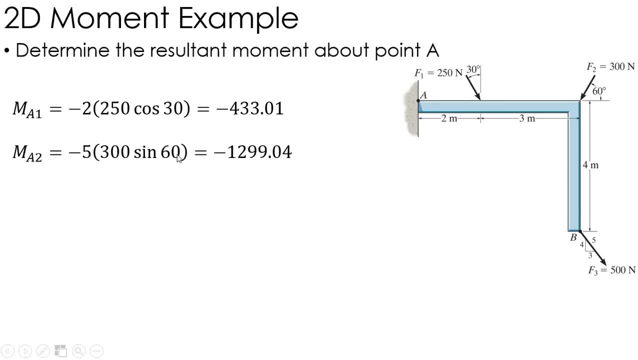 So I get negative 5 times 300 sine 60. That's the component or the moment of the 300 newton force about point A, And that's negative 1300 newtons or 1299.. Now this final force. I'm going to break it into its two components. 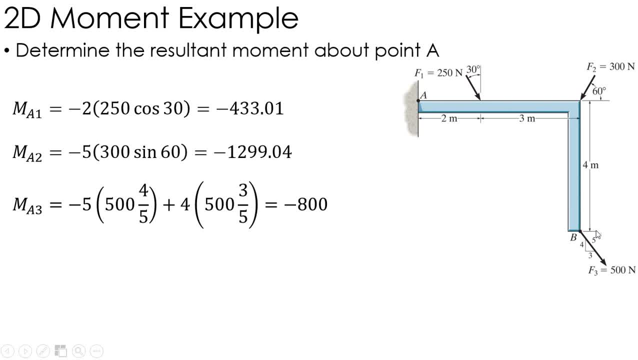 I've got three-fifths times 500 horizontally And four-fifths times 500 vertically. Now both of these components are creating a moment, So we'll start with the vertical component, That would be the four-fifths times 500.. 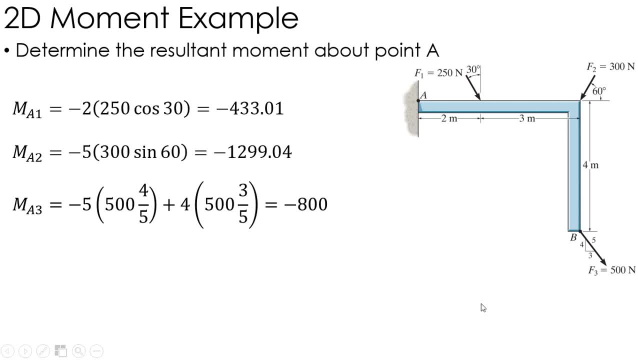 It's going to be five meters away. It's acting down. That creates a clockwise rotation. a negative moment about point A, So I would have negative 5.. Again, that would be the five meters Four-fifths Times 500.. 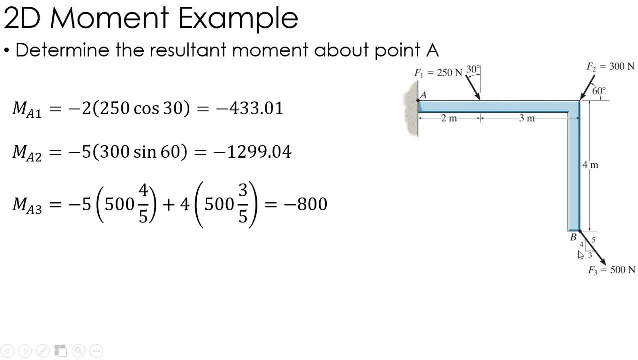 So I go negative. 5.. Four-fifths times 500.. Now the horizontal component, that's the three-fifths component, That is a perpendicular distance of four meters away. Now, this moment, heading to the right creates a counterclockwise. 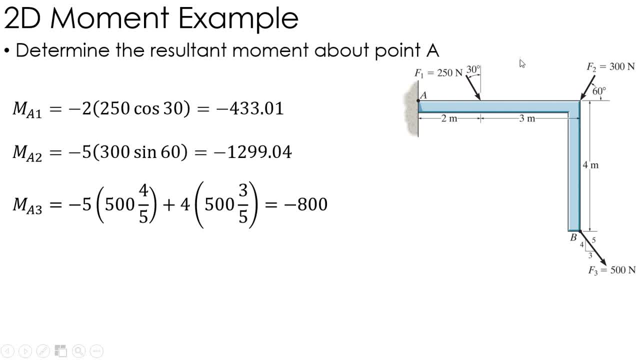 Rotation about point A. That would be a positive moment. Counterclockwise is a positive moment, So it's pushing this way. It creates a positive moment about point A, So that would be positive. perpendicular distance of four meters times three-fifths of the 500..